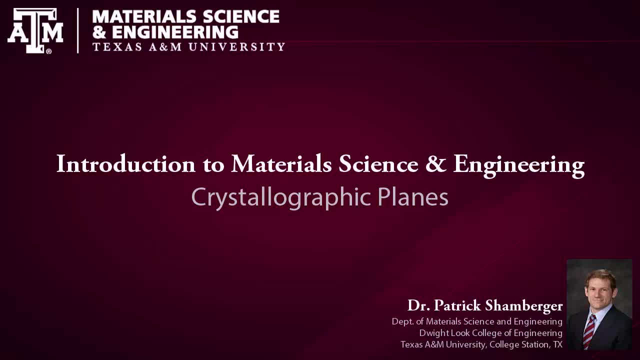 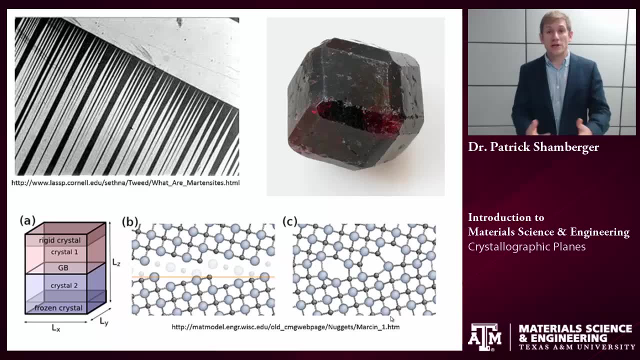 Howdy. The point of this video is to discuss how to index crystallographic planes using the Miller indices. So why do I want to describe a plane? Well, there are lots of two-dimensional features, surfaces, interfaces, boundaries and crystal structures that I would like to. 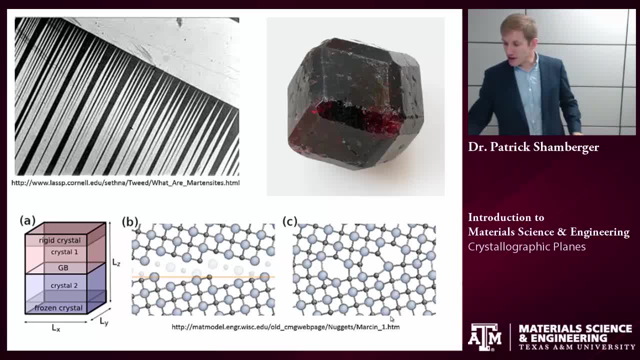 be able to describe and define. Here are a couple of quick examples. If I'm looking at martensites, so this is twinning in a martensitic structure and the twinning is observed along very specific crystallographic planes in a structure. Another example would be if I'm 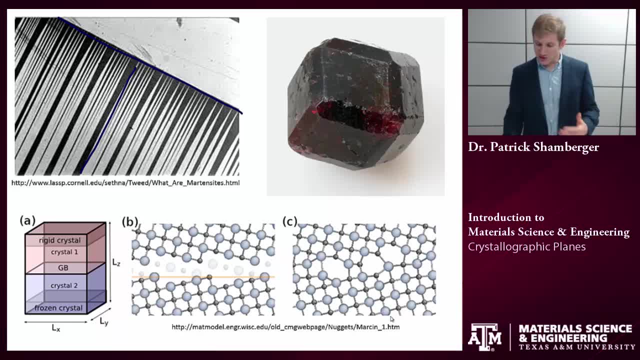 looking at the grain boundary between two neighboring crystals. So that is the interface separating two individual crystals, each with their own unique orientation. Finally, if I want to describe crystal habits, So these are free planes in a single crystal, as the crystal is growing. So if I want to, 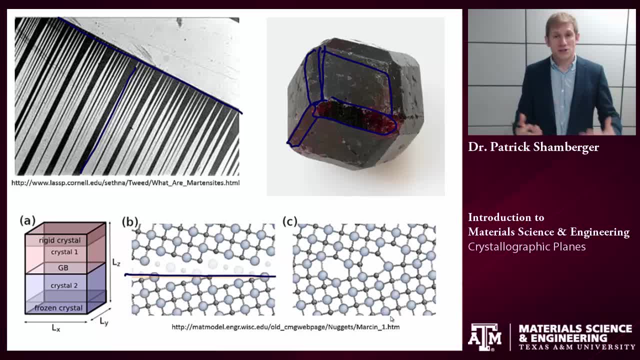 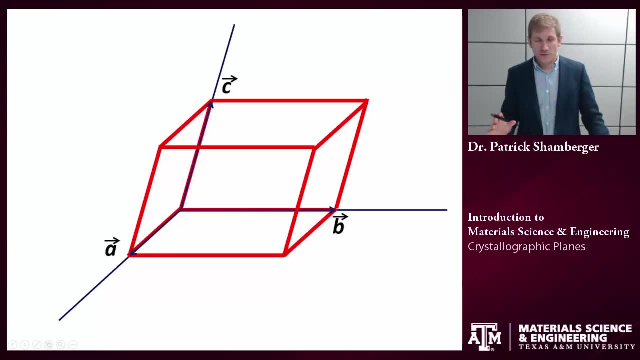 describe these surfaces, I also need to describe them in terms of crystallographic planes. We do this using the Miller notation, So let's try some examples. We're going to start off with a general triclinic axis, so three lattice vectors different lengths and not perpendicular to each other, Say I have 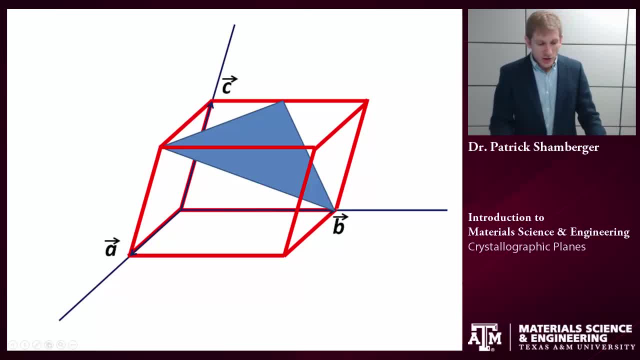 this particular plane that I want to describe. So there are basically three steps that we need to do to index a plane: We need to look at the intercepts, We need to take the inverse And we need to reduce any fractions. Okay, what do these steps mean? Step number one: 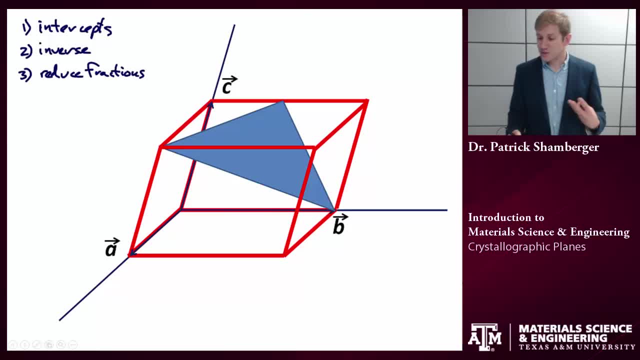 intercepts. Where does this plane intersect with the three principal lattice vectors? What are the fractional coordinates of those intercepts? So this is pretty obvious for one of them, For B, it intercepts at one, But it's not so clear where it intersects the A and C axes. And this is: 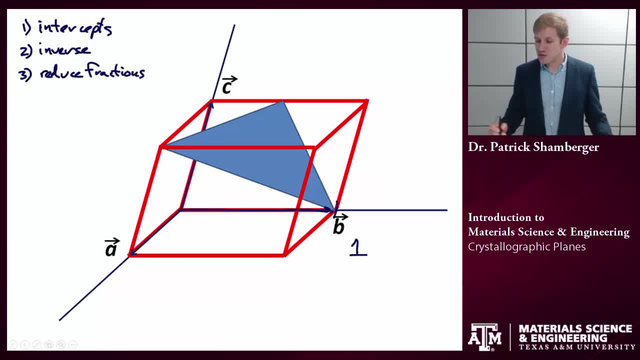 generally the case For the plane that's illustrated in some unit cell. you might need to extend that plane to figure out where it intersects these axes. So we're going to do that. I see that this line here. if I kept extending it would intersect the C axis up at 2.. Similarly, 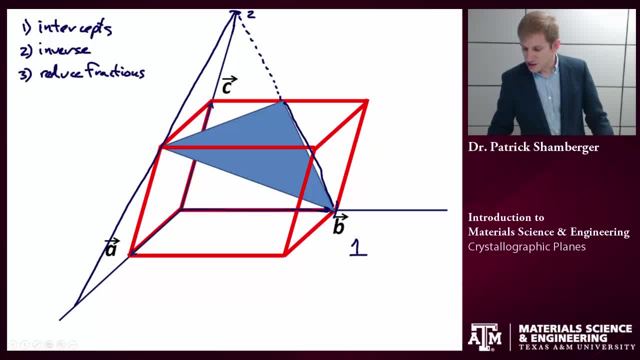 I need to draw an extended line here, Or I could come from this side Passing through one half, And I see that it intersects the A axis also out here at 2.. Now, this might be a little bit hard to visualize, So take a moment and try and work it out for yourself. 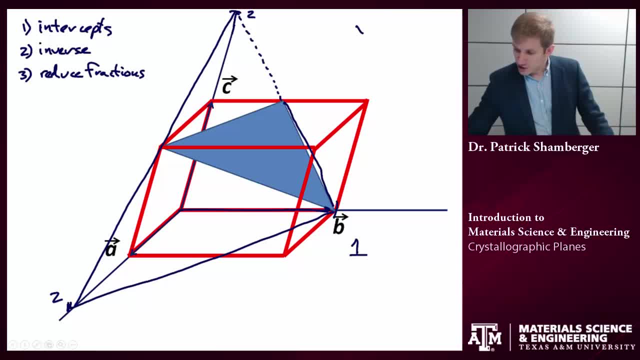 So I know the intercepts. I would encourage you at this point to start with a table. The intercepts here are 2, 1, 2.. The next step is to take the inverse of those: One half 1, one half, So 1 over 2, 1 over 1, 1 over 2.. Now this is kind of tricky and this is 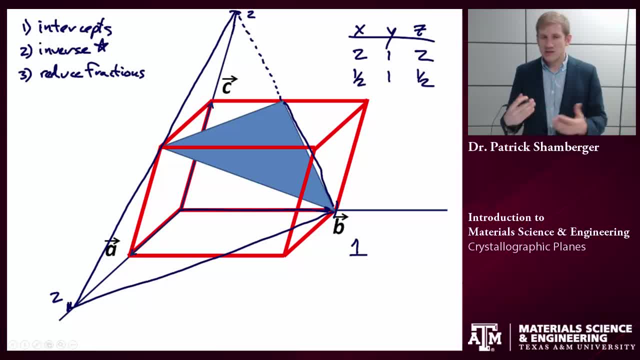 often times what people forget: When we're doing directions, we don't take the inverse at all. When we're doing planes, we do take the inverse. When we're doing planes, we do take the inverse. So students often times confuse the 2. So just a word of caution. 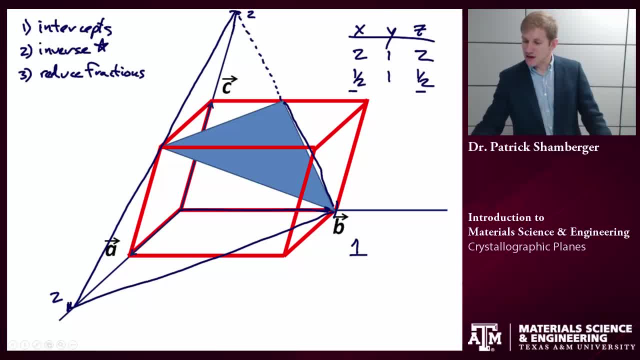 The third step is to reduce the fractions. So here we see fractions. I'm going to multiply this all through by 2. And I'm going to get 1,, 2, 1.. So I have to multiply all 3 of these. 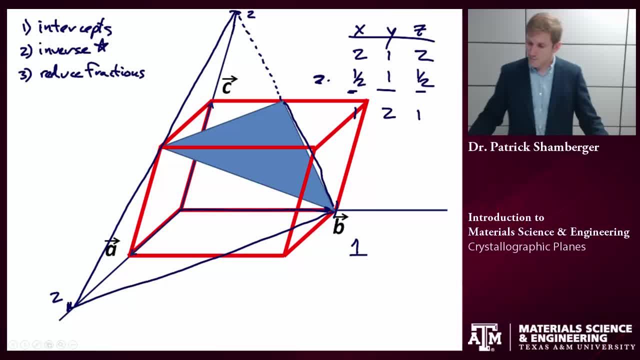 numbers through by the same number in order to reduce the fractions. And if I were to write this in the standard Miller notation for planes, that is 1,, 2, 1.. I don't use commas and I use round parentheses, So a single plane is described by round parentheses. 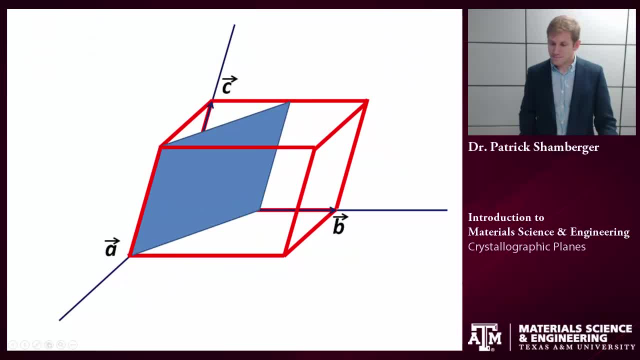 So these are the Miller indices of this particular plane. Let's try a different case, and this is going to show us one tricky thing you might encounter. So again, my three steps: Find the intercepts, find the inverse and reduce the fractions. So I'm going to write this: 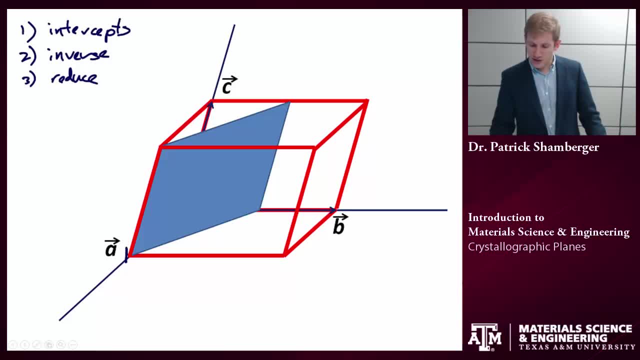 here. So what are the intercepts? It's intersecting A over here at 1.. It's intersecting B over here at 1 half, But it never intersects C. So this plane is parallel to the C axis. In this case, I would say that the intersect is at infinity. And to convince yourself why, 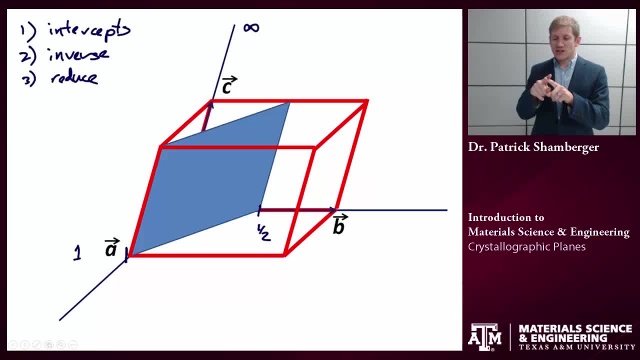 that is, think of two planes that are not parallel, but I'm rotating them so they're getting closer and closer to parallel. As I do that, that intersect point is going to get further and further away, And so when they are actually parallel to each other, 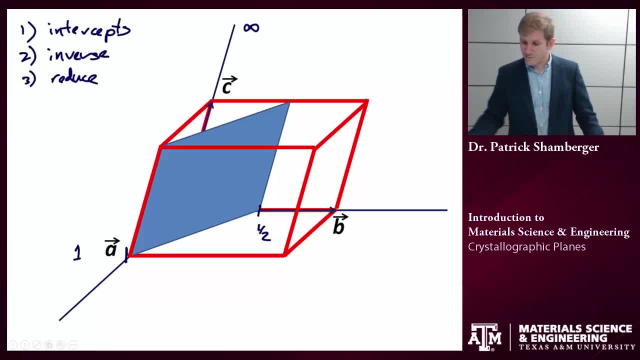 they never intersect or that intersect point is at infinity. So in my table x, y, z, the intercepts are 1, 1 half infinity. I'm going to take the inverse of these. It's the next step. 1 over 1 half is 2.. 1 over infinity equals 0. 1. 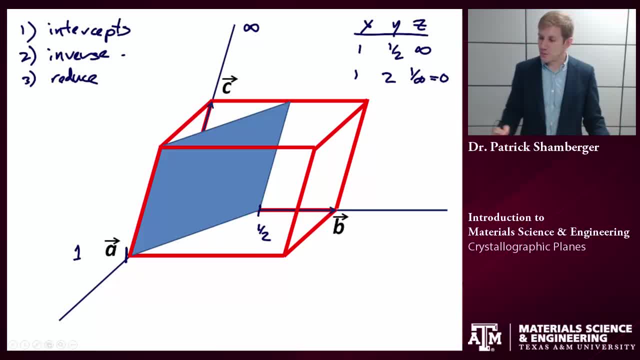 divided by an infinitely large number is 0.. I would then reduce, but I notice I'm already using integers only. So I'm all set. The indices of this plane are 1,, 2, 0, using the Miller notation. So note, if I'm parallel to the C plane, my C index is going to be 1,, 2, 0. 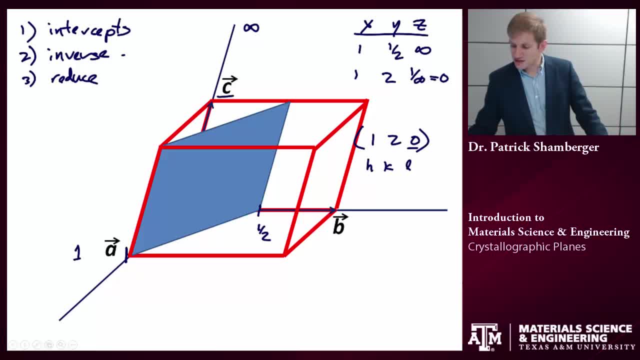 I've set the C for 1 and 0, and 2 for infinity. I'm all set for infinityIntercept vector x, 1 and 2, taking the property again the C, into infinity. This double K plus. 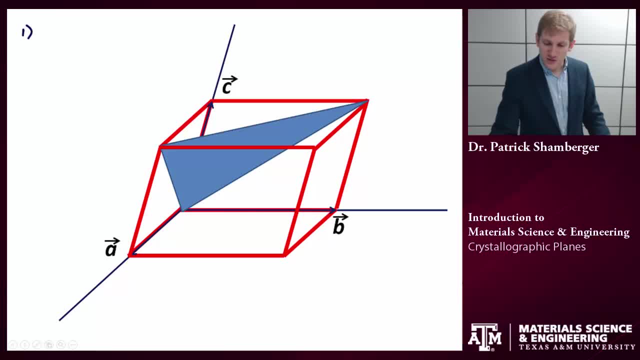 L into infinity is 0.. These are actually usually called H K L indices, So the L wouldn't be 0.. Let's try another tricky one again. I'm always going to use these same same steps. I take the Minecraft to therus And then I reduce my fractions. So where are the intercepts in this case? Well, to me it looks like it. intercepts a beingization equals a power minus a. So clean up any reading you have in this class. You can add, Or the line you want in the window, which is always one: add to do what you make of it as a justınız, a zwTOR. 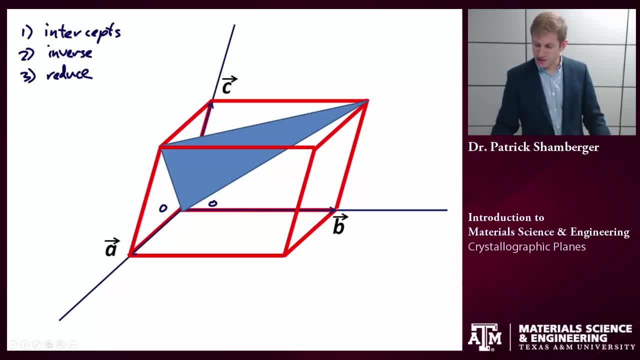 at zero, it intercepts B at zero and it intercepts C at zero. So if I were to take the inverse of zero, zero, zero, I'm gonna get infinity, infinity, infinity, and this is not a really well-defined plane. 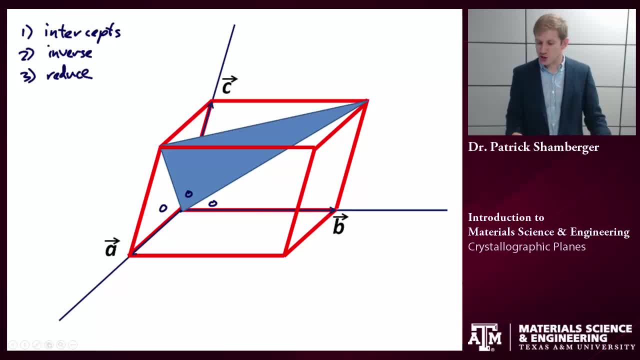 So the problem is that I'm passing through the origin. So anytime the plane is passing through the origin you need to do something to figure it out. You can either move the plane in the unit cell or you can move the origin. The two are identical. 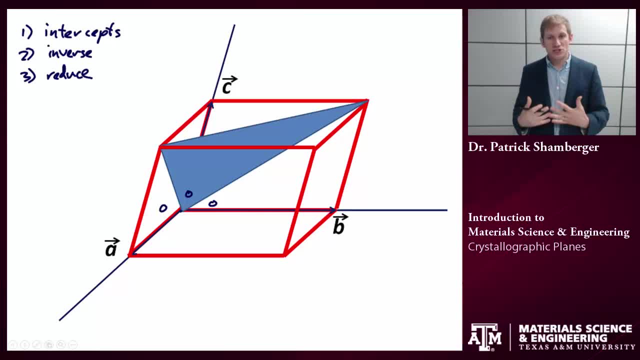 Again, when you're indexing planes, just like directions, the absolute position does not matter, It's just the orientation of this with respect to the origin. So I am going to shift the origin so it's up here in the back left upper corner of this unit cell. 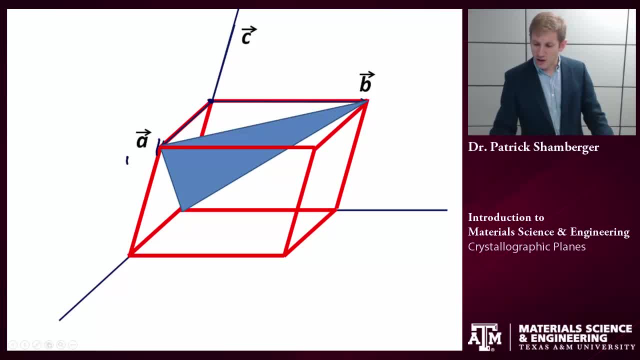 So again, I'm gonna take the intercepts. It intercepts A at one, it intercepts B at one and it intercepts C at negative one. So if I write my table, I have one, one negative one. The next step would be to take the inverses. 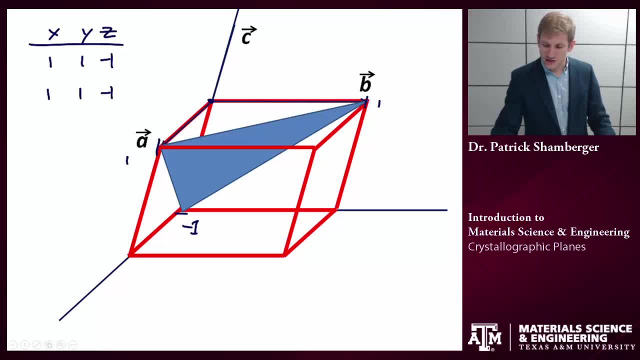 but the inverse of one is one, the inverse of one is one, the inverse of negative one is negative one. So I don't need to do anything. I also don't need to reduce, because these are all already integers. So the Miller indices for this particular plane. 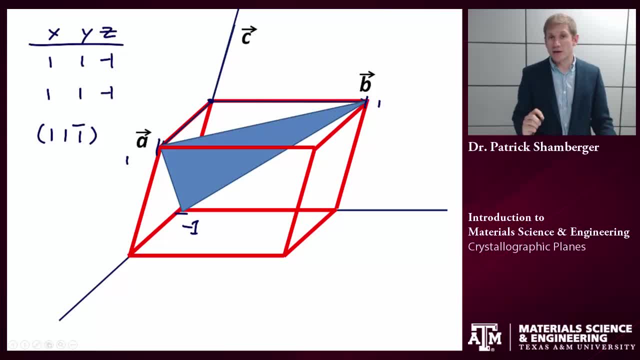 are one one, bar one, So this is pronounced bar one And this is the notation Notation, crystallographic notation- for negative one. Usually it's written like this Sometimes when your professors are giving you homework assignments or making tests: 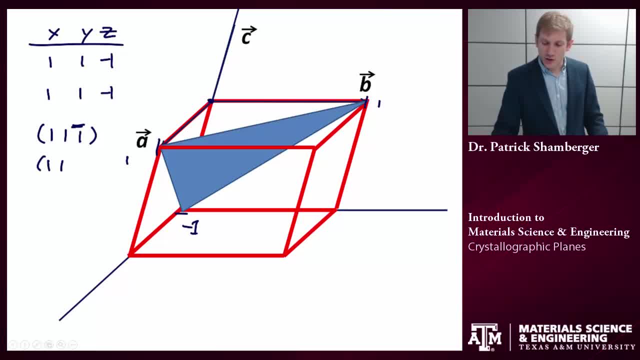 it's tricky to get that bar in exactly the right place. So they will write something like this with the negative one sign, But the proper notation is one one bar one. Okay, the next kind of a challenge would be if you were given the indices and asked to draw a plane. 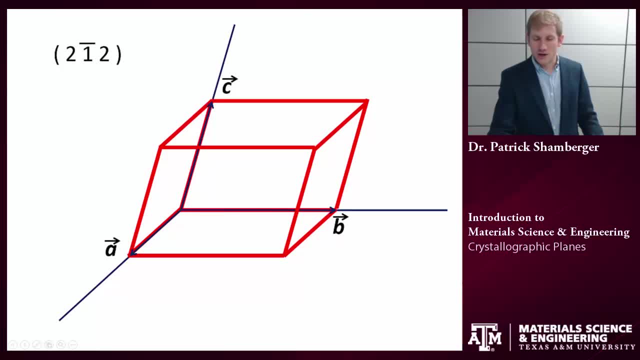 So here we're given hkl of two bar one. So again that's negative. one and two. Now, because this is a negative number, I know one of two things are gonna happen. Either I'm gonna be intercepting somewhere. out of the unit cell off in the negative direction. Well, that is gonna happen. So the alternative would be to redefine to shift our axis off to this side. This is, you don't have to do this, You can just extend your unit cell outwards. 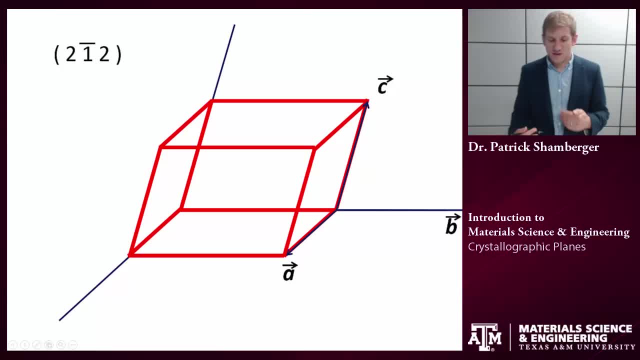 I find this to be easier sometimes, So we're gonna do the exact opposite of the process from before. So I know the final notation. Essentially, I need to take the inverse of these. So the inverse of this is one half negative one, one half. 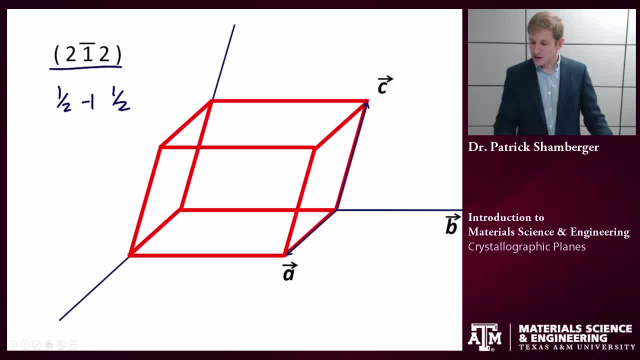 And then these are now the intercepts. So the intercept with the a-axis is one half, The intercept with the b-axis is negative one, And the intercept with the c-axis is one half, And so this plane is going to look like this: 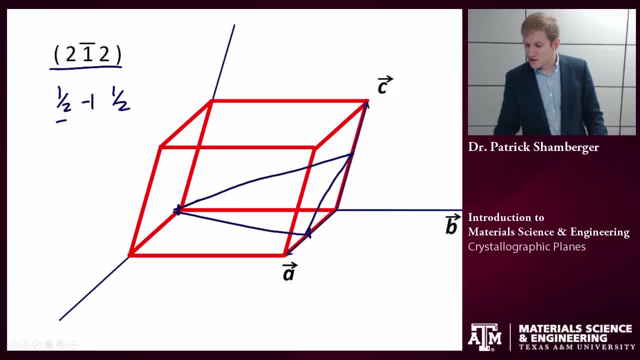 Again, you only need three points to define a plane And because I shifted that origin at the beginning, it's a little bit easier because now it's all falling within that original unit cell. So with planes, remember that second step, taking the inverse.